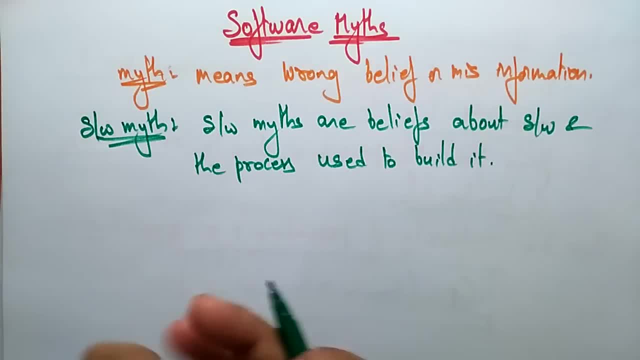 So here, the software myths are just beliefs about the software that we are using and the process use it to build the software. So in those areas our beliefs will be there in the view of different people: in the customer view, in the management view, in the user view, the development view. 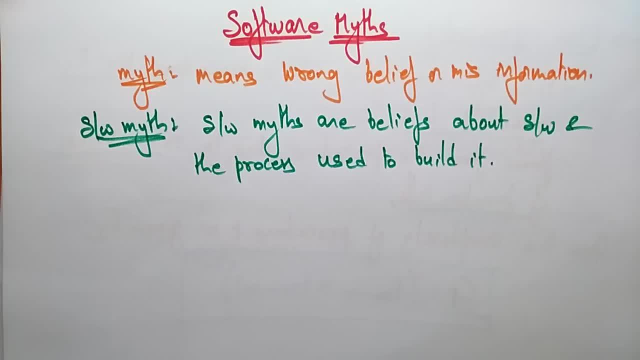 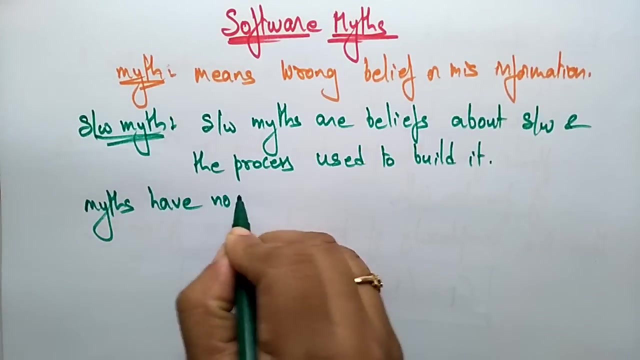 So every person is having their own software. myths means their own beliefs about the product or the process and about the software. So that is about the software that you call it as a software myth. So the myths have number of attributes. that causes serious problems to the software. 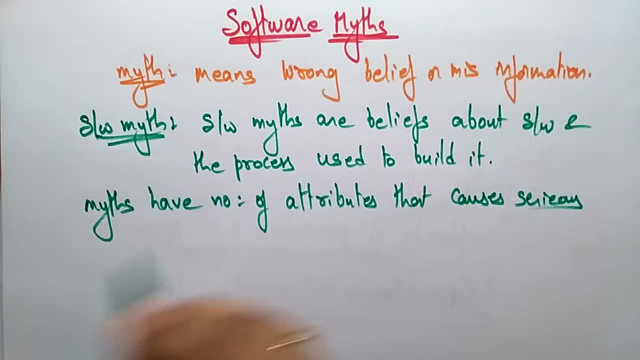 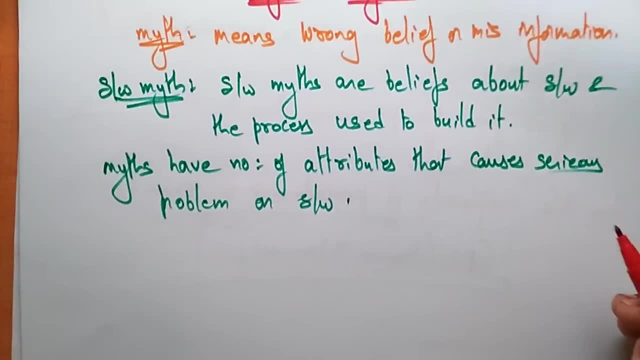 That causes serious problems on software. So actually there are three types of myths will be present. totally, they are there. So actually there are three types of myths will be present. There is no explanation for it. There is no technical explanation for it. three types of myths: one is management myth, customer myth, and the third one is developer or practitioner myth. so these are the three different types of myths. now let us see one by one. so what is that? let me explain about the customer myth. what is the customer myth? 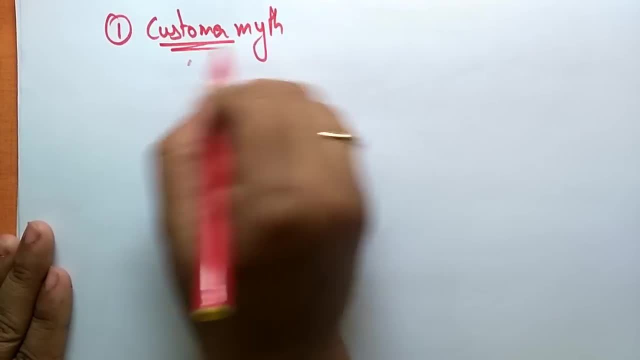 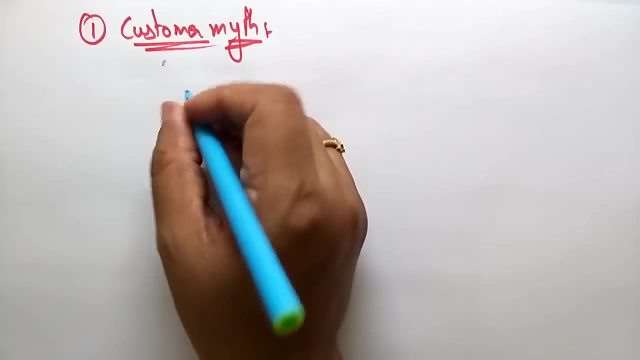 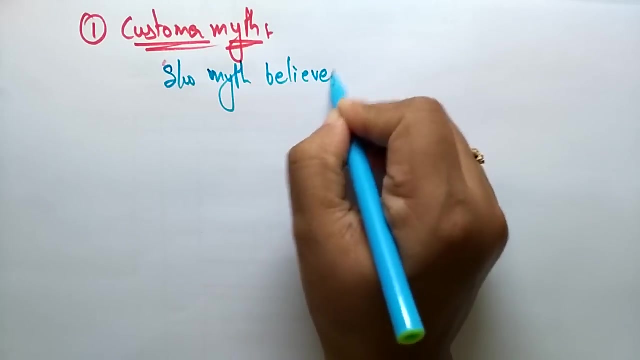 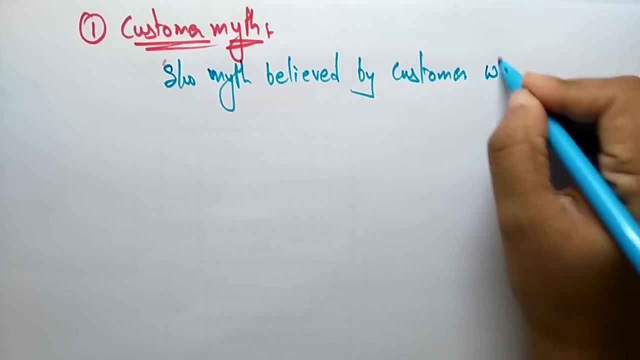 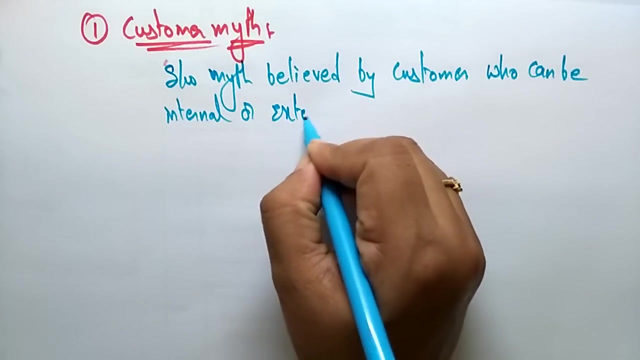 what is a believer, that the customer will always think about the software or the process. actually, the software will always think about the software myth here in customer view, the software myth believed by customer who can be internal or external, who can be internal or external? so what the main? 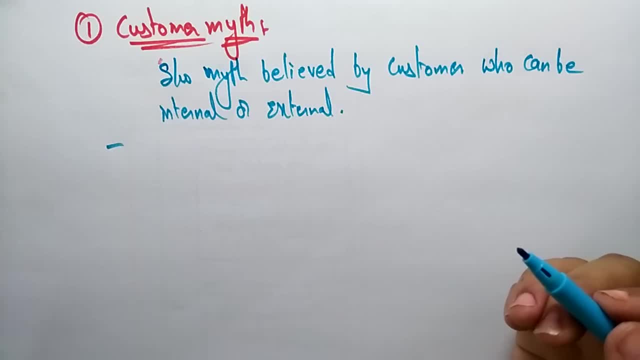 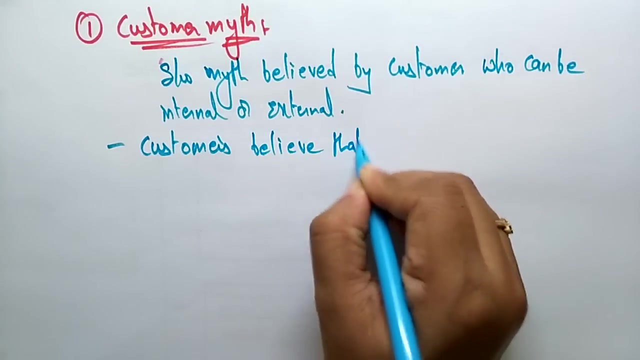 the customer will think about what is his belief about the software, so what the customer myths about the software, about the process they are using to build. so the customer believes, customers believe that general statements of objectives is sufficient to begin writing a program. so whatever the general statements that are present, 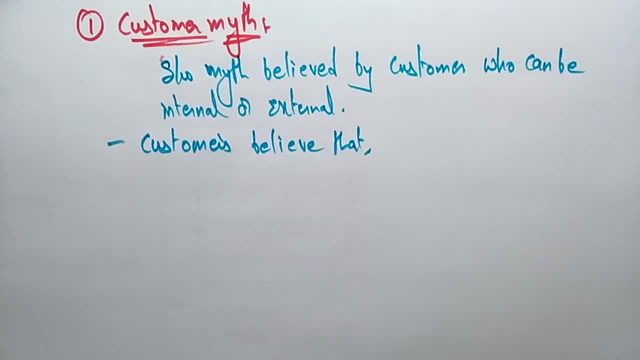 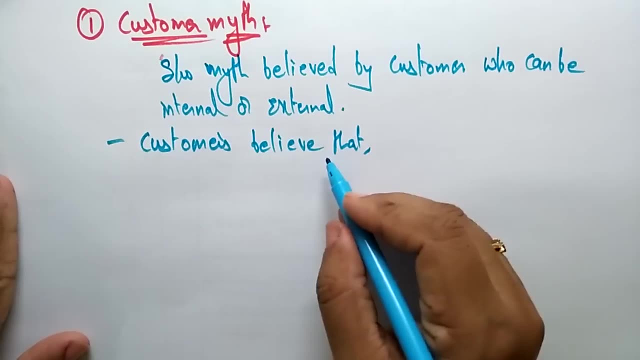 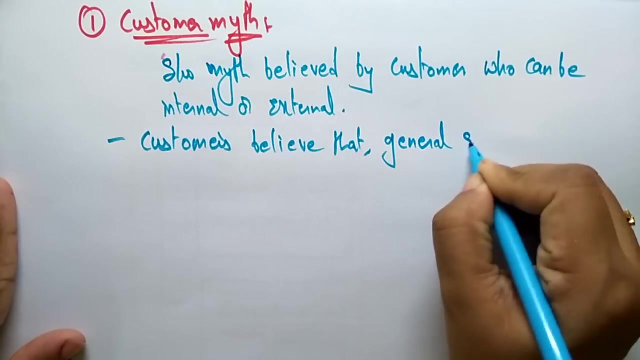 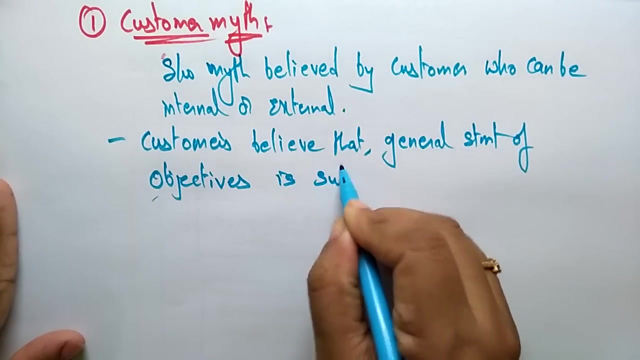 up to so far. now, those are enough to write a program, he may believe. so that is only the belief. ok, that you call it as a myth, always as a customer myth. in the customer point of view point of this, the customer believe that general statement of objectives is sufficient to begin writing the program. so to write the 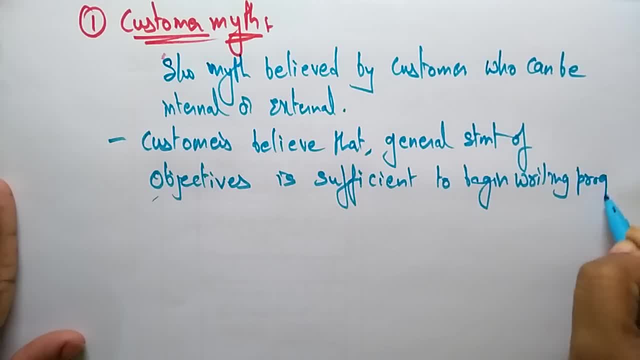 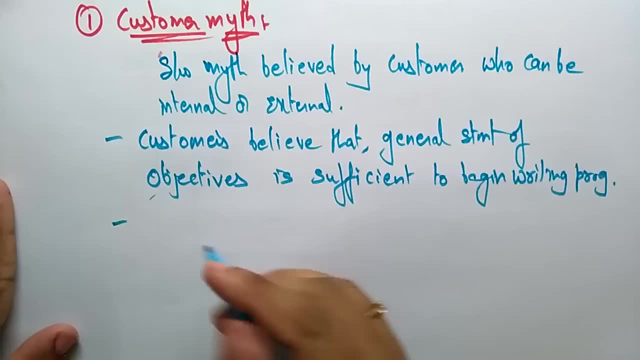 program, some small, sufficient statements or enough he may think he believe, and the requirement changes are easy to accommodate. because the software is flexible. he think that changing requirements is sufficient. change requirements always. changing the requirements is easy, the software is, so the customer is thinking that he is believing that changing the requirements 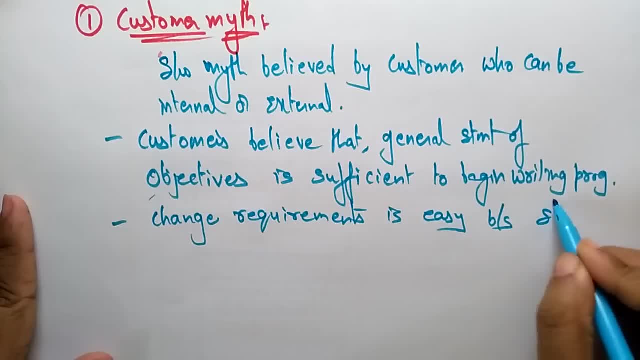 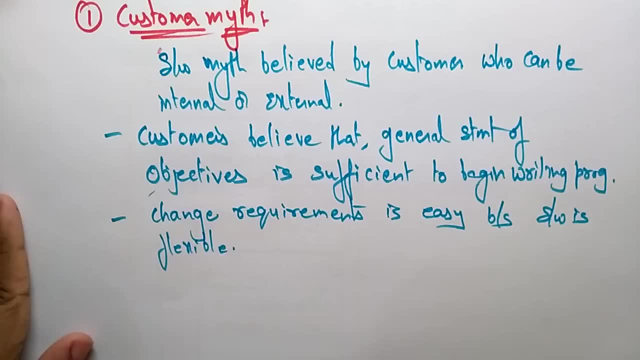 is always easy because software is a flexible. he may think that the software is a flexible. it is a belief. it is a wrong belief. okay, you can say it is a wrong belief about the product, about the customer developers, about the company they are giving the project. okay, change in requirements is easy because 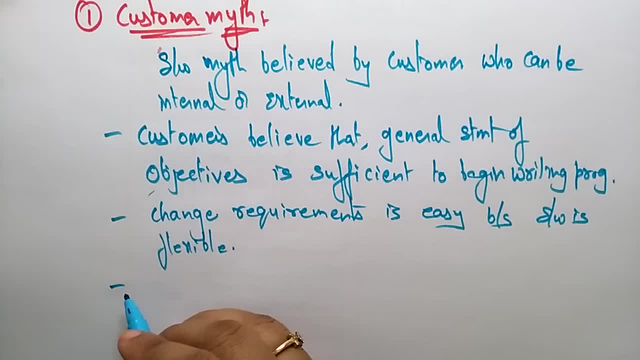 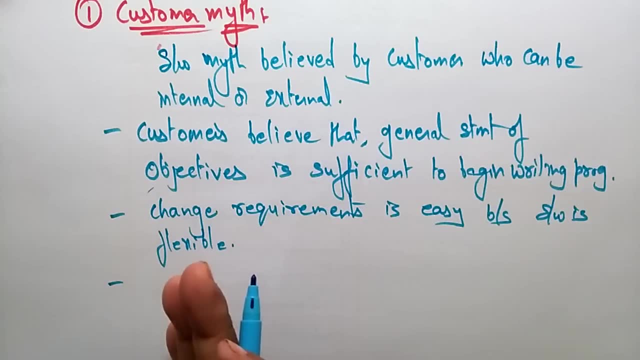 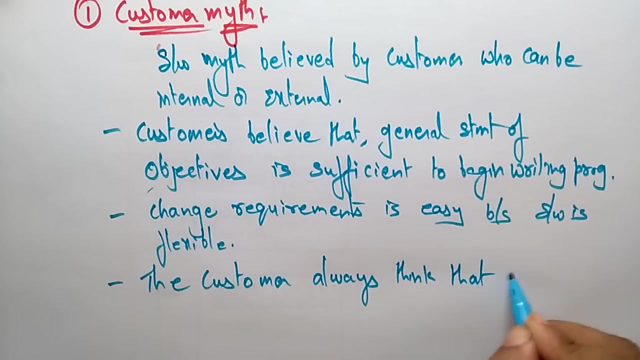 software is flexible and another myth: he is thinking that this is everything. this is primarily seen in evident because the client always think that software development is an easy process. the main thing is: the customer always think. a client always think that the customer or a client always think that software development 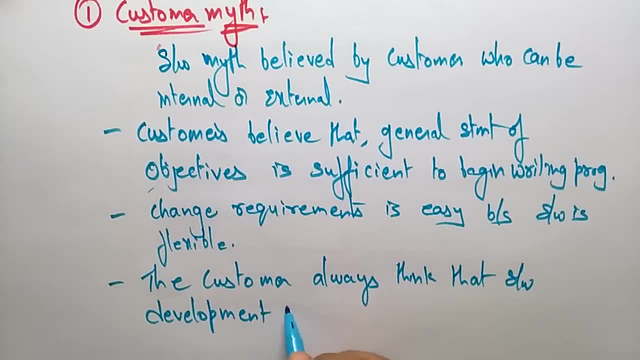 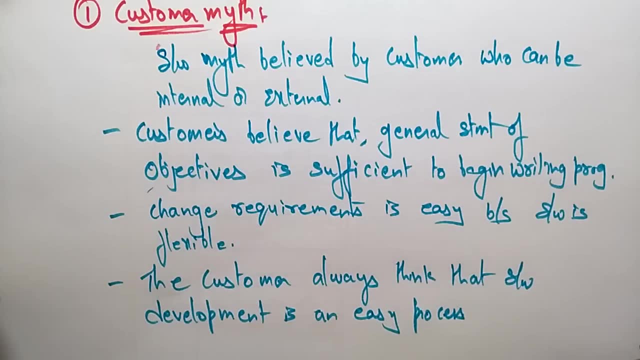 is an easy process. actually, the person who is going to be implemented, he knows the pain of creating the product. he creating the code, creating the software, but the cost in the view of the customer, made they are. these are all the beliefs of the customer while they are giving the project. 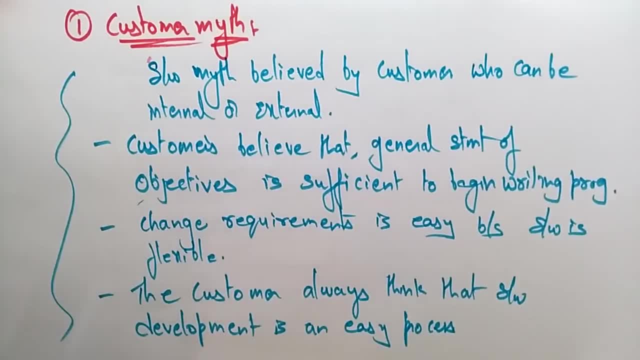 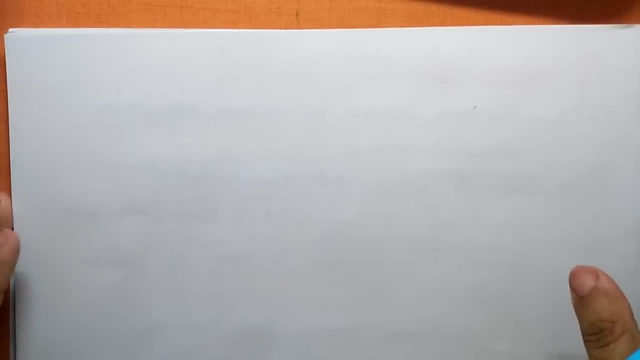 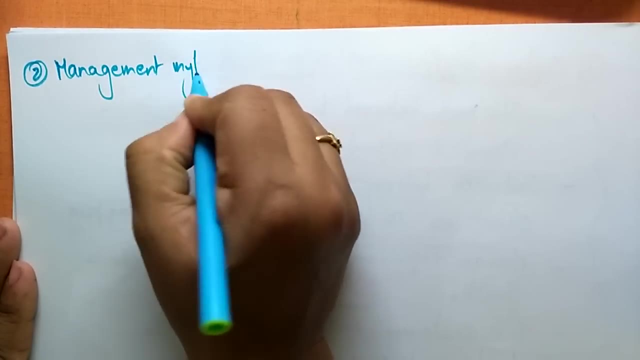 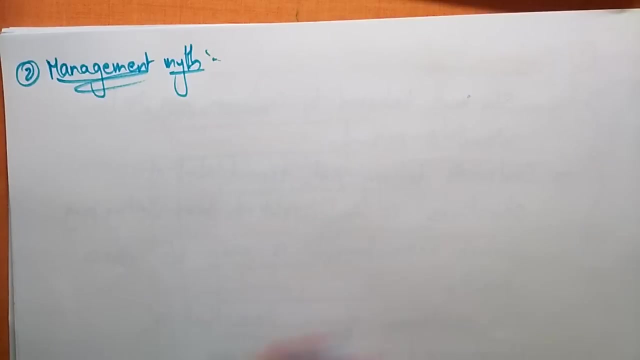 to the company or any organization. so this is a customer. now let us see what is the management myth. what do you call this management? okay, so let me explain about the management myth. you, so management make means uh, here we have standard, we have some standard uh, and processes for building. they are the management people, what they believe. 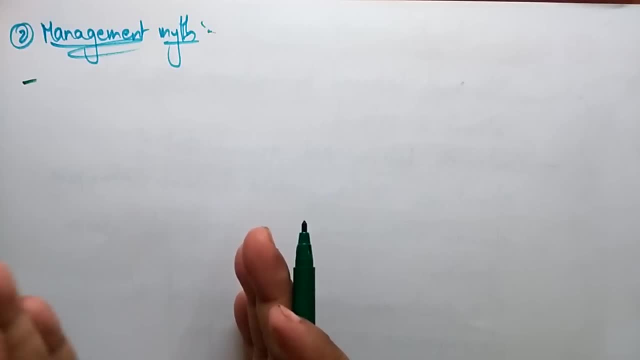 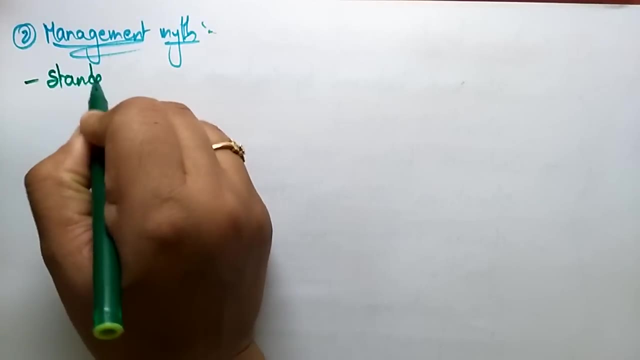 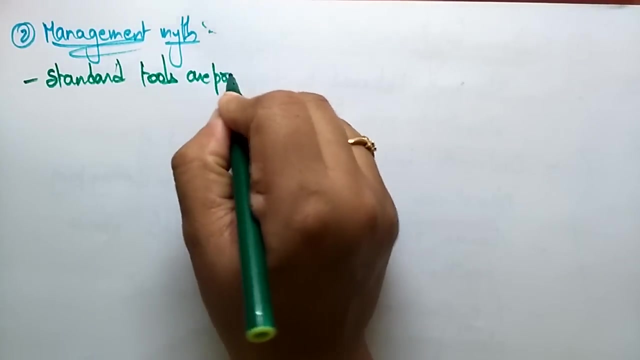 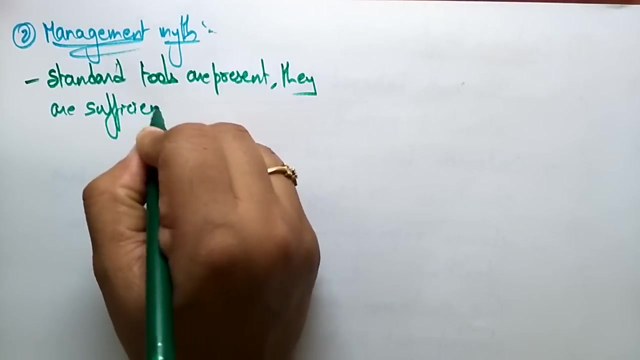 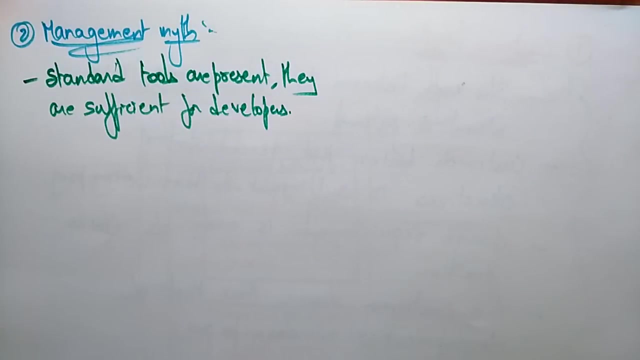 they believe that some standards and procedures were for building software is enough, so developers have everything they need to know. okay, they thought that some standard, standard tools are present and they think they are sufficient. they are sufficient for developers to develop the program means they are believe the management belief is whatever, whatever it present. 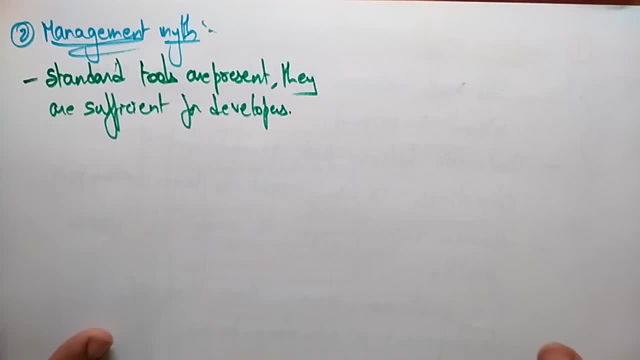 so far here in the company, those are enough to develop a project. but what we can say internally? the developers may need some extra tools to develop a project. okay, but the management believes those are enough. if we are behind schedule, we can. the another management myth is they can think that if you are 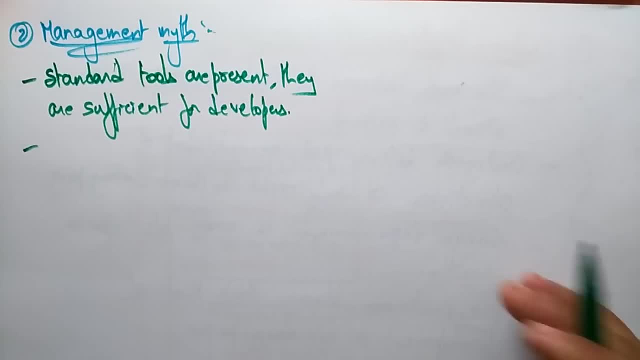 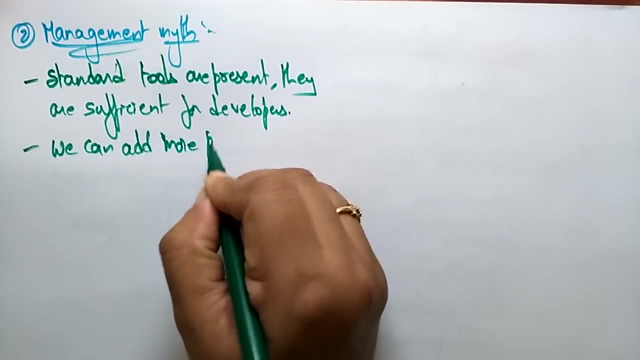 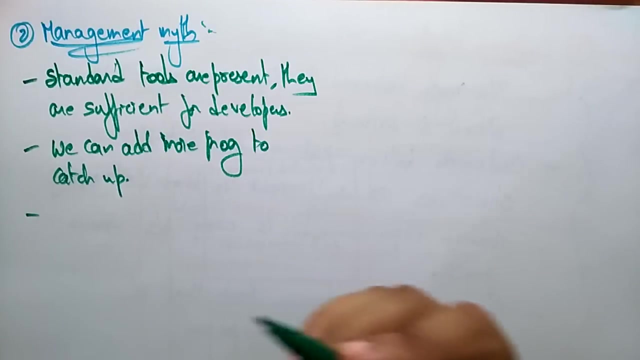 behind schedule. we can add more programs to catch up. so they thought that we can add more programs. okay, more programs to catch up. it's just, they believe the management belief and they think that we have state-of-art software development tools. after we all, we buy this latest company, they think that they will always. 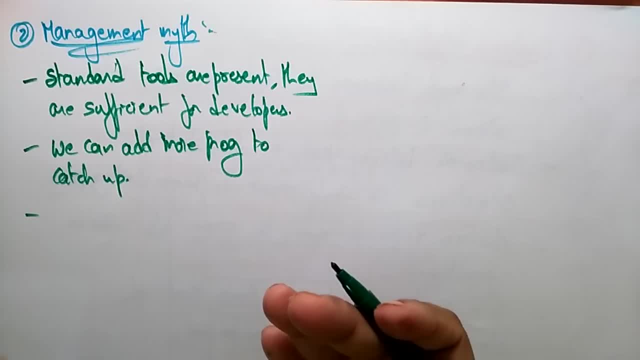 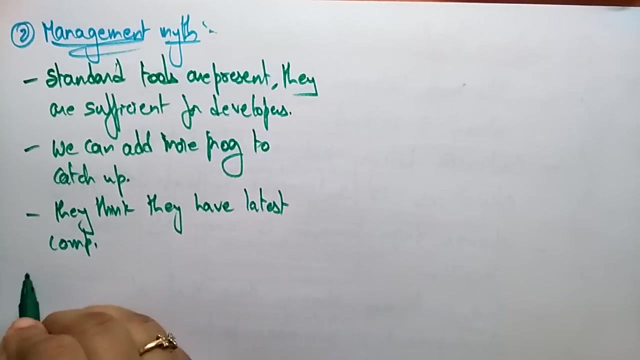 believe buying the latest component computers, so it is sufficient. they think that there is a management method. they think they have latest computers. actually the usually the myth of manager was he think always a good manager can manage any project. a good manager can manage any project. so this is about the management. 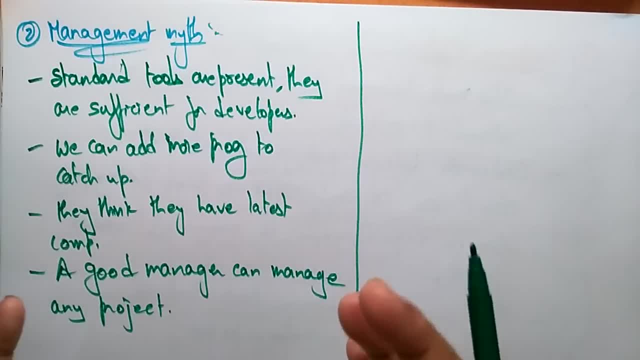 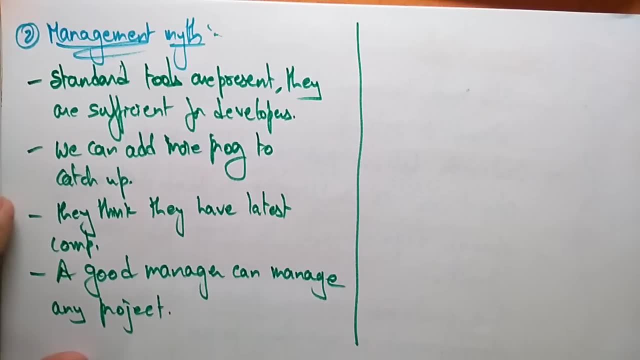 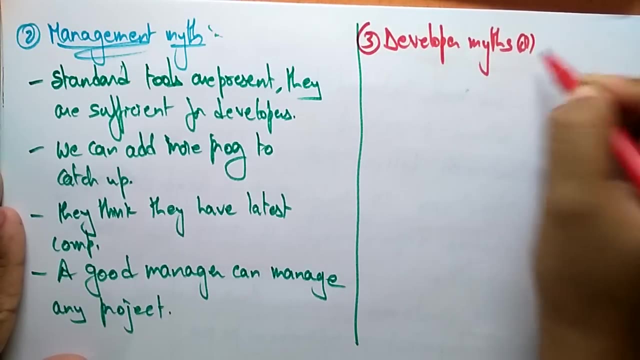 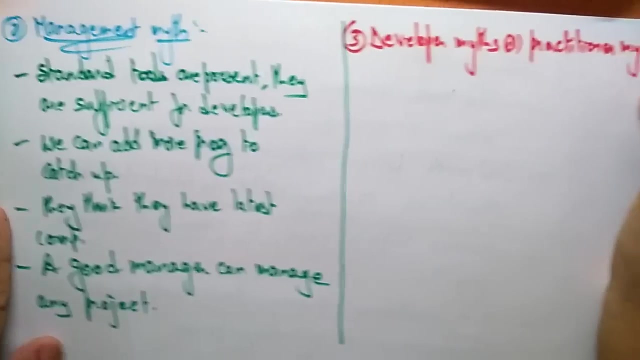 myth, the management belief. okay, so the software myths are divided into three types: the customer myth, management myth and the developer myth. now coming to the third one, that is, the developer myths, or you can call it as a practitioner, myth, practitioner. it is a developer myth or a practitioner, so what the developer believes, what he think. 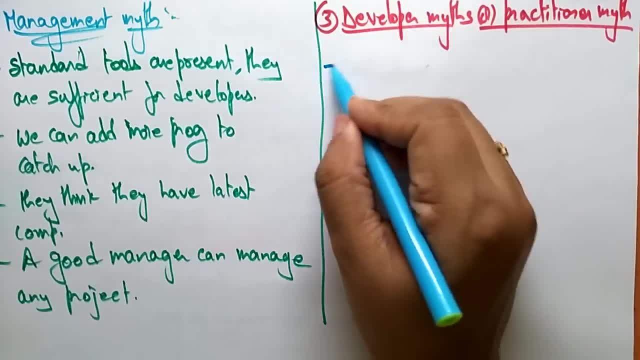 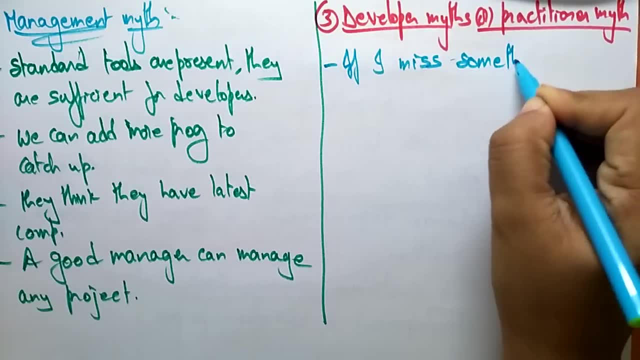 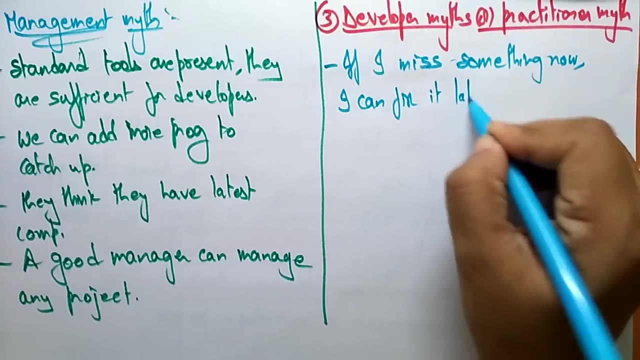 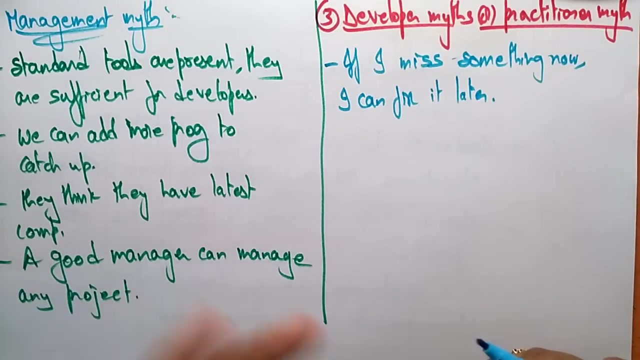 about the software. so the developer, they think, if I miss something, I miss something now, I can fix later. his next like negligency, because he, whenever he is writing the code, he know that he's miss something. okay, even though I miss something, I can fix it later. because if 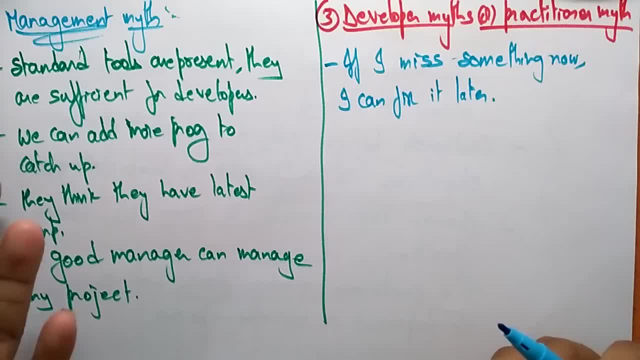 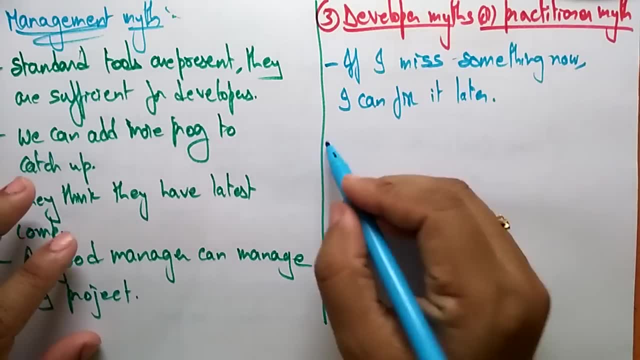 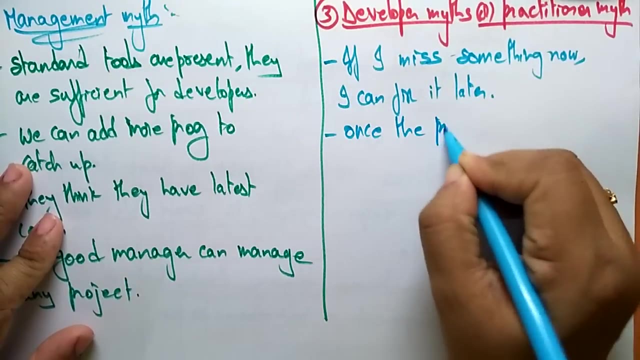 raining and no, no error will come, it will be soared. if error will come, then we will think about that, means they believe they believe that, okay, we can fix it later. that is so. they think that if I miss something now, I can fix it later, once the program is. 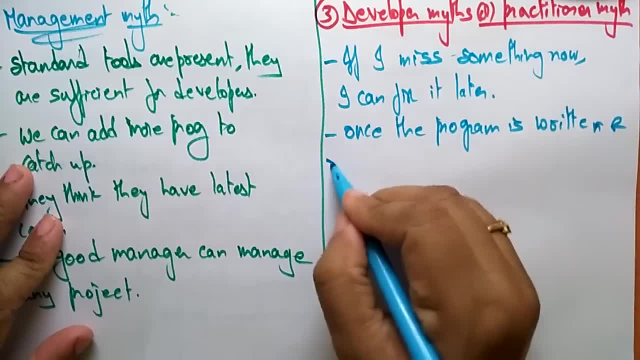 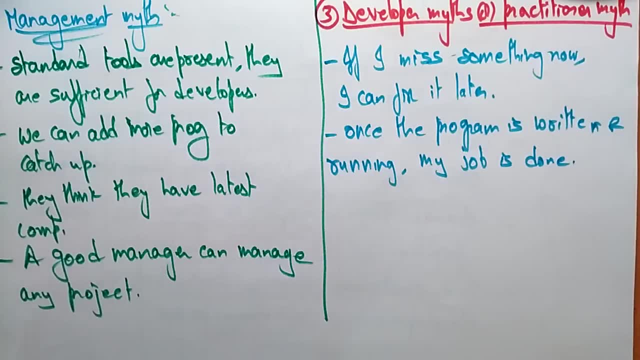 and running my job is done. so he think that, okay, once i written the code, okay, today's my work is over if it is running. the code is running, okay, my job is done means he is just believe that he is not, uh, fully dedicated. means he is just doing his work. he thought that that whatever he done is a 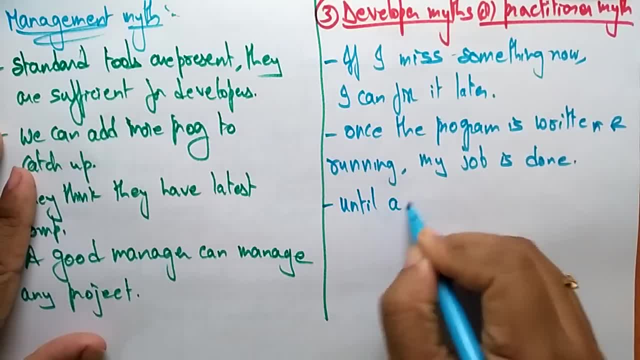 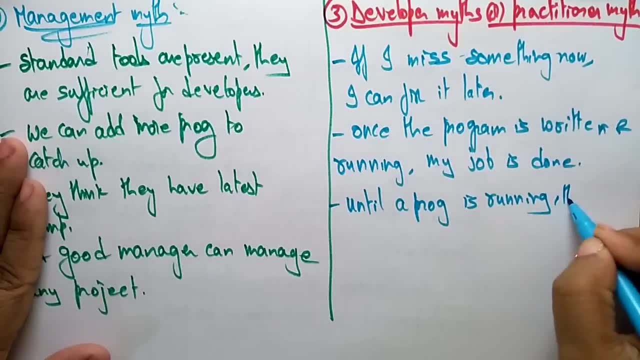 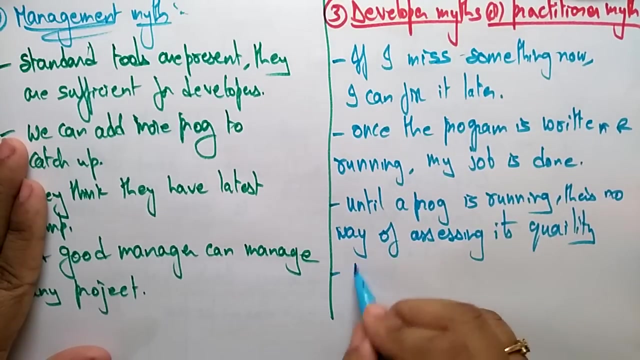 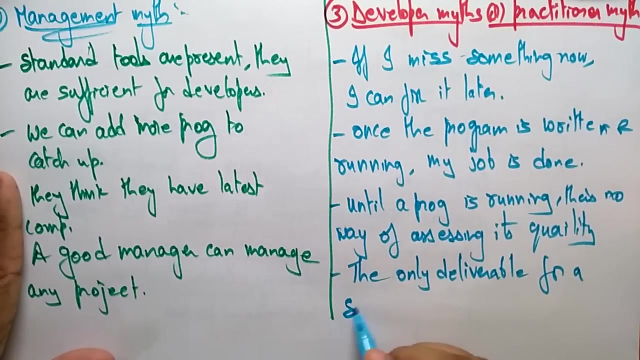 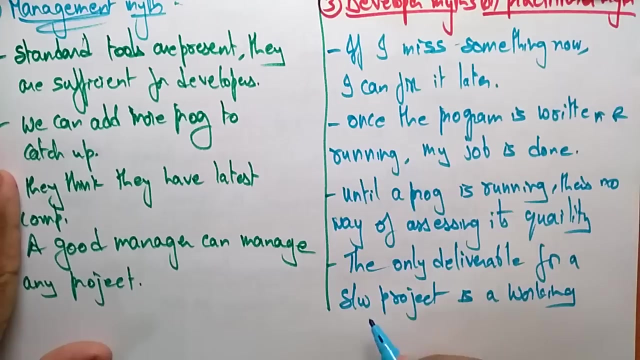 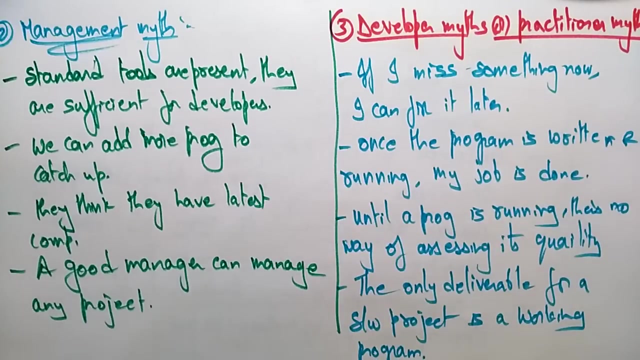 correct until a program is running. until a program is running, there's no way of assessing its quality. so this is also his belief. and next, the only deliverable, the only deliverable, deliverable, the only deliverable, the only deliverable, the only deliverable For a software project is a working program. The main thing he will think is: whatever the program, that software I going to be delivered, that should be in working. So it's just beliefs. So these are all the three different types of software myths. 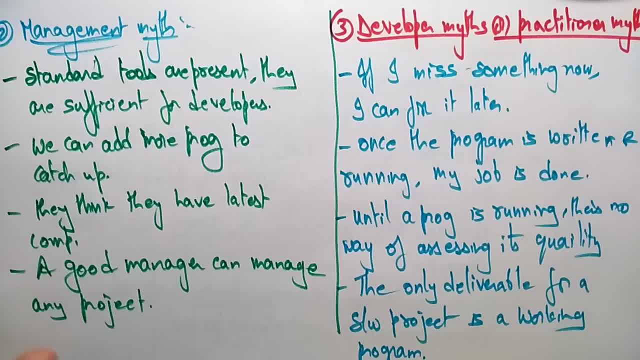 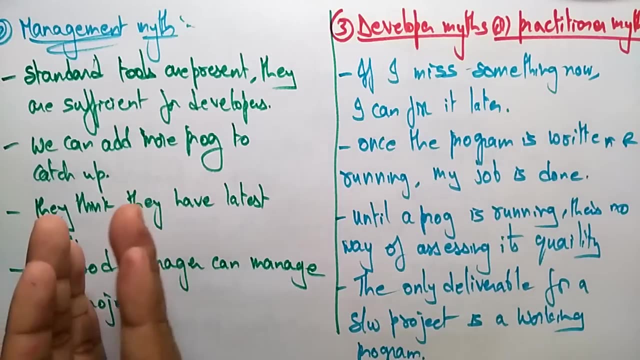 One is the customer myths, management myths and the developer myths Means in those way views, what they think about the software, what they think about the company, the customer, what they think about the software, what he think about the management and the developers. and the management myth. 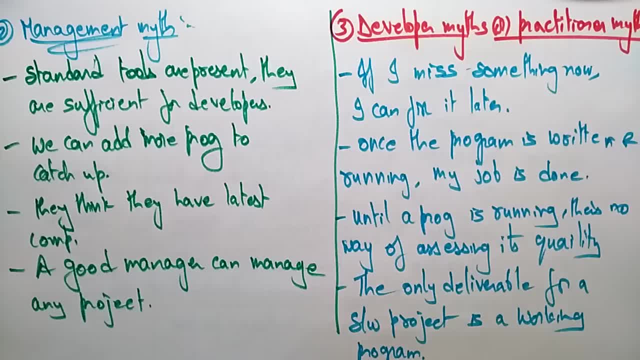 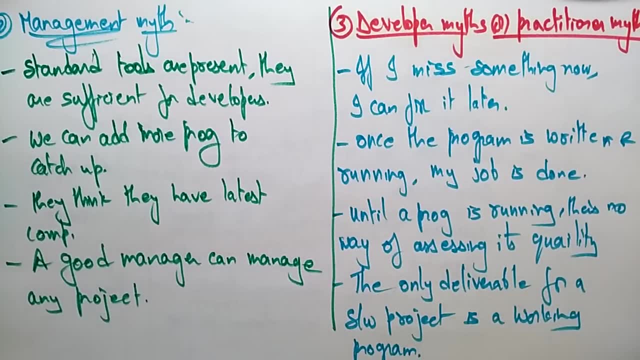 So what he thinks about the company and what he thinks about the project, what his beliefs and, in the view of the developers, So what he believes about the project. That's it, Thank you.